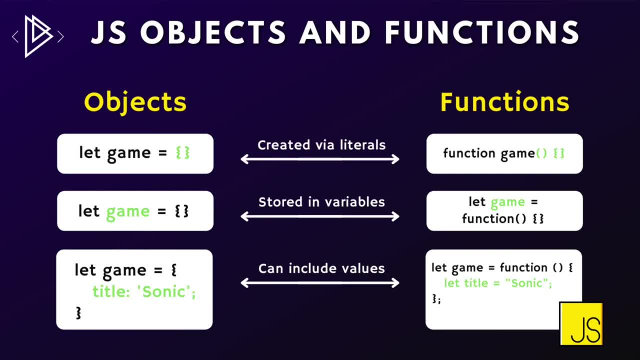 Objects can be stored in variables. Functions can be stored in variables. We can include conjunctions that can be used toでは tuntattip, a character in a sentence. Speedpen needs to allow you to Movie. We don't want to use the value function as a definitions to use it. 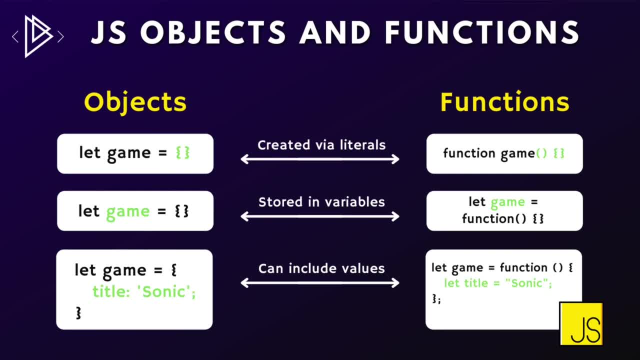 include properties and values inside objects and we can do the same in functions. Remember, the data type for a function is an object. we learnt that way back in our lesson on data types in lesson 7. I believe The key difference between an object and a function is that with 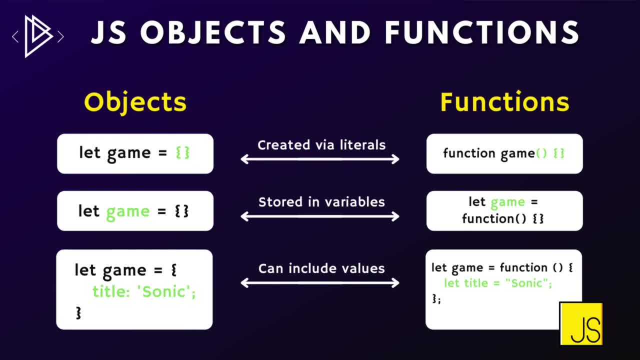 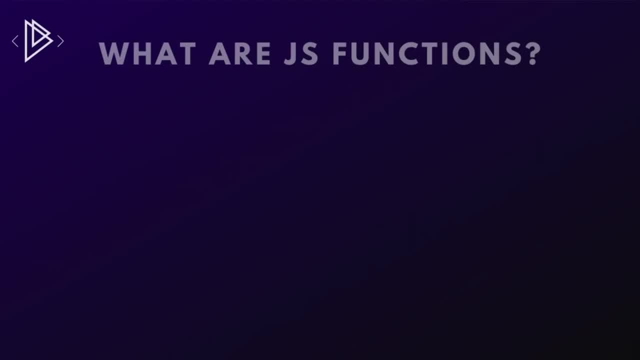 a function. we can call or invoke a function. Now, right now, that probably doesn't mean anything to you. so let's first understand what are functions and then we can understand what we mean by calling or invoking them. So functions are blocks of code that we can call, or the. 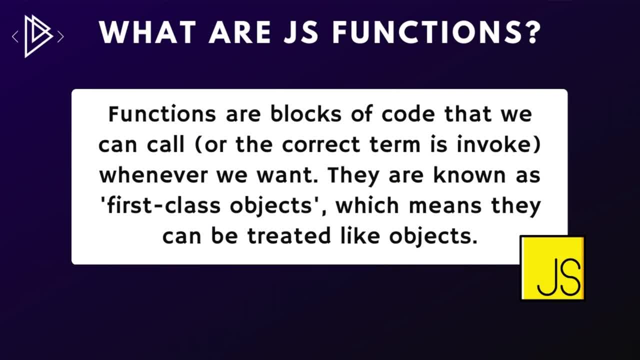 correct term is invoke- whenever we want. They're a key part to JavaScript's power and expressiveness, and in this first lesson on functions, we're going to learn all about how to write functions and their basic usage. So the first thing to know about functions is that they are first. 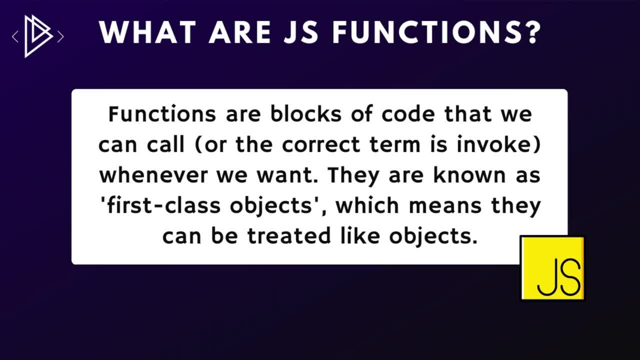 class objects. This basically means that they coexist with and can be treated like any other JavaScript object. They can be referenced by variables declared with literals, etc. etc. So that's what functions are. they are blocks of code that we can call or invoke whenever. 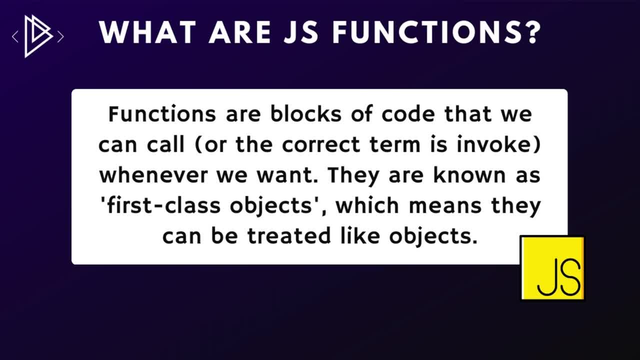 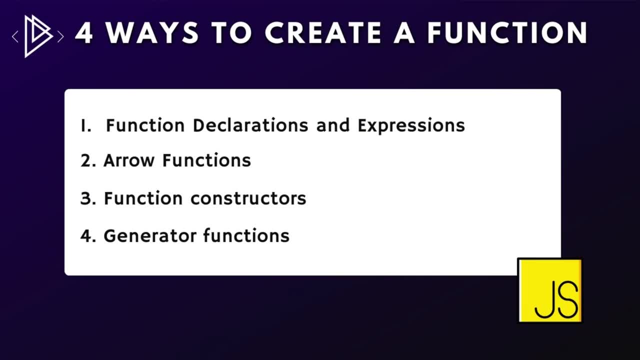 we need them. So that's all about what functions are. Now let's take a look at how they can actually be created. So there are four main ways that we can create a function: Function declarations and function expressions. These are two of the most common ways to declare a function. 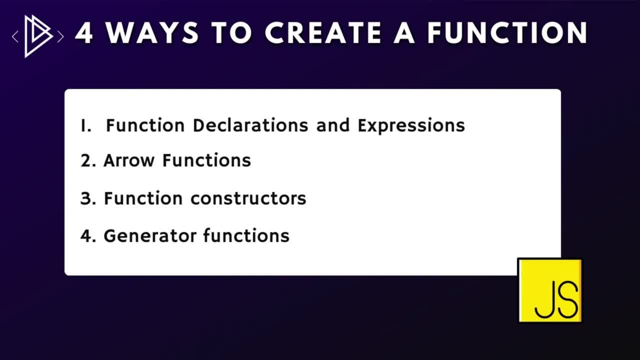 and we'll be looking at function declarations in this lesson. Another way that we can create functions is by using arrow functions. Arrow functions were introduced to the language with the ES6 update. They're a cleaner and simpler way to declare functions, but they're 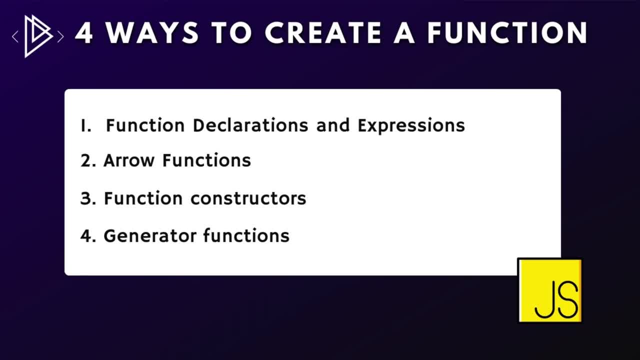 not just there to look pretty Arrow. functions solve a very common problem for us when it comes to creating functions and, of course, we'll take a look at this when we look at our functions later on. The third way to create a function is a function constructor. Now, function constructors are: 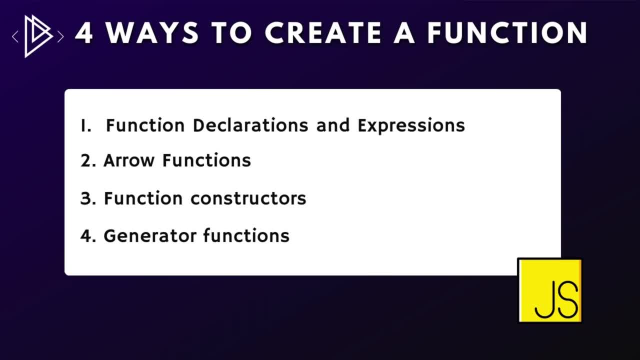 very rarely used odds are. you'll never use them, and so we won't be discussing this in a lot of detail. I will probably touch upon this later on, just for completion, but we probably won't be going into it in a lot of detail. 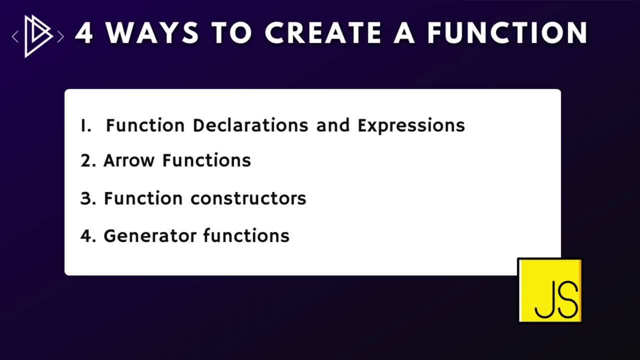 And finally, the fourth way to create a function is by using generator functions. Now, this way of creating a function can be rather complex. Essentially, generator functions allows us to create functions that can be any number of times. So, for example, if I want to create 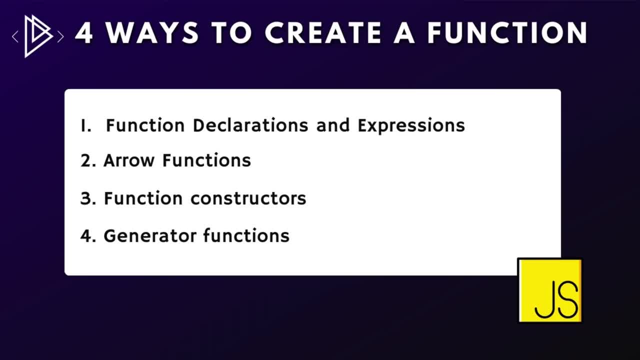 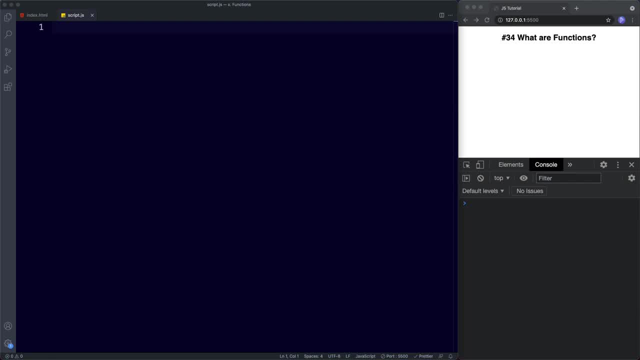 a function that can be exited and re-entered later, something we can't do with normal functions, So we'll look at these later on in detail. Okay, so that's enough theory, then, So let's start then with creating a function declaration. 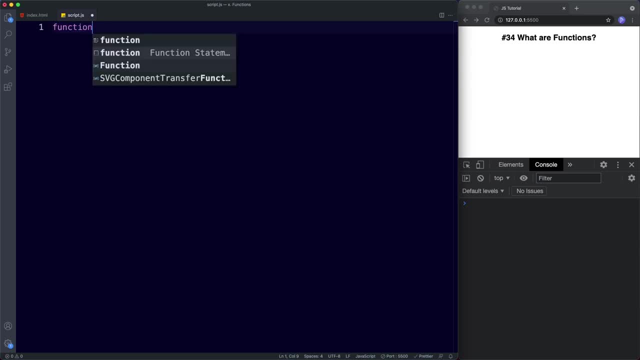 So in here I'm going to simply use the word function space, and now we need to name our function, So I'm going to call this function games. Next we have a parentheses space, curly braces, and inside here we'll have our code that we 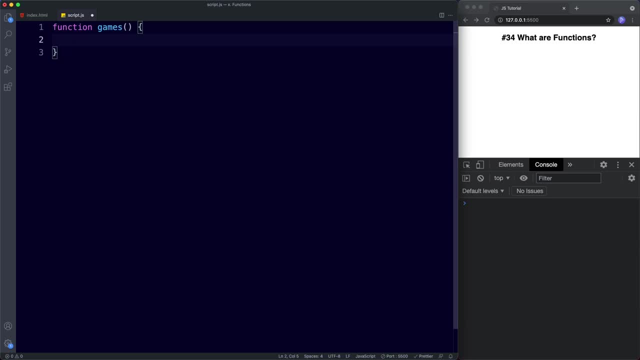 want to call or invoke. So this is the basic syntax for a function declaration. We have the word function space, then we have a name for our function. Immediately after the name we have parentheses space and then curly braces. So inside this I'm just going to consolelog a few things. So I'm going to say consolelog. 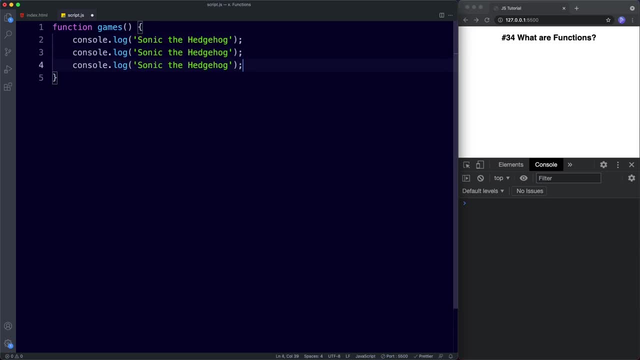 Sonic the Hedgehog, and we'll do two more consolelogs. We'll say consolelog Super Mario and for the game, let's go for Donkey Kong. Okay, so we've created our function declaration, So we use the keyword function, we name our. 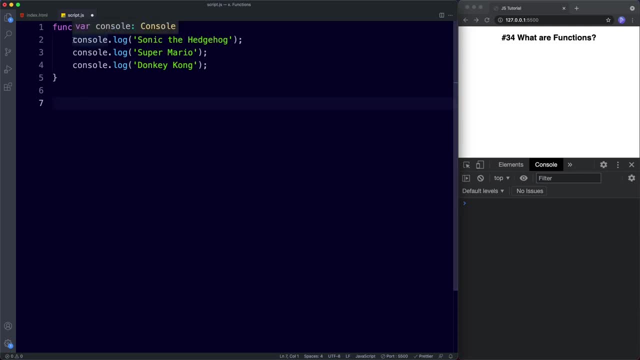 function, parentheses, curly braces. and inside our curly braces we have our code to be run. So how then do we actually call or invoke this? Because if we save, notice that nothing happens. We don't see this in the console. So note that simply creating a function doesn't. 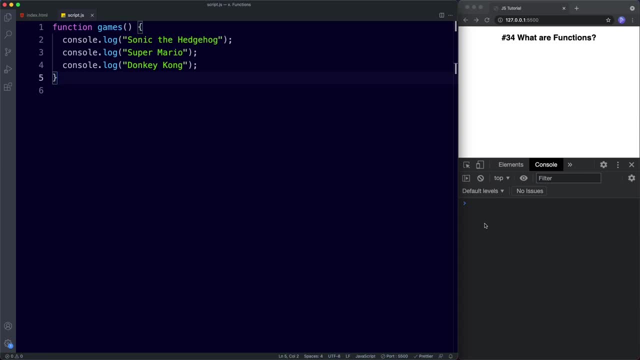 actually run any of the code. To do that, we must call or invoke the function. So the way that we do that is outside of our curly braces. now We simply use the function name. so it was games- and then- very important- we include the parentheses at the end. Now it's actually. 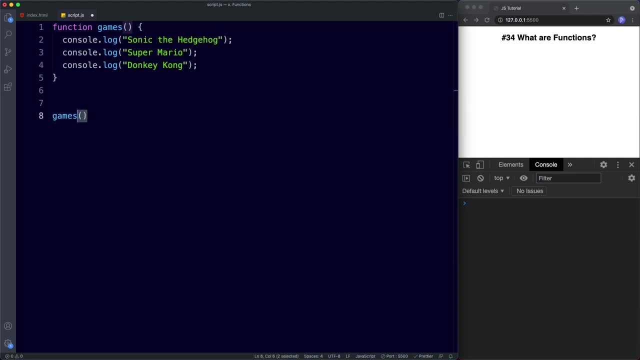 this parentheses here- that is responsible for calling or invoking this function. If we simply said: games like this and let's save, nothing happens. Once again, very important to know: it's the parentheses that actually invoke the function, So let's save this now. 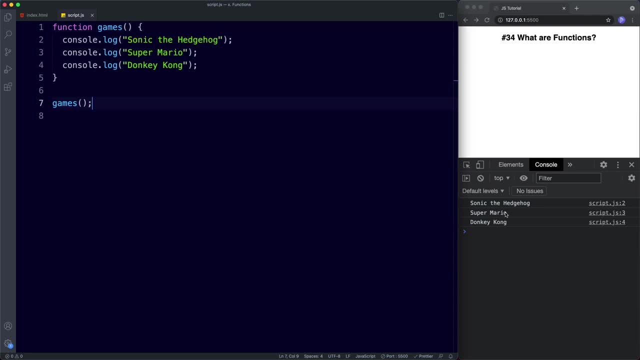 And now, you see, in our console we have our three games: Sonic the Hedgehog, Super Mario and Donkey Kong. So this is great, We can call this whenever we want. So if we were to repeat this a few times and save, we get. 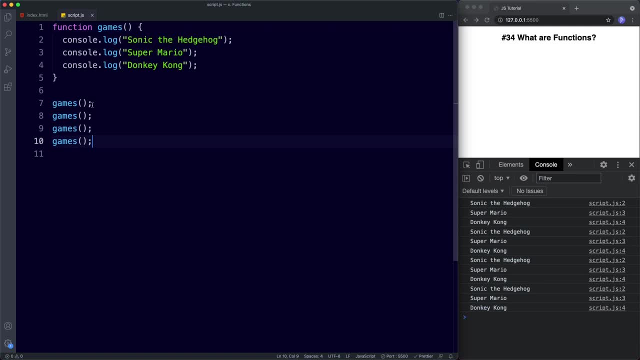 our console logs multiple times because this function is being invoked multiple times And if we go back to one function call, our code is executed once and we get our console logs So already. then we can see a big advantage to using functions Any time we want to run. 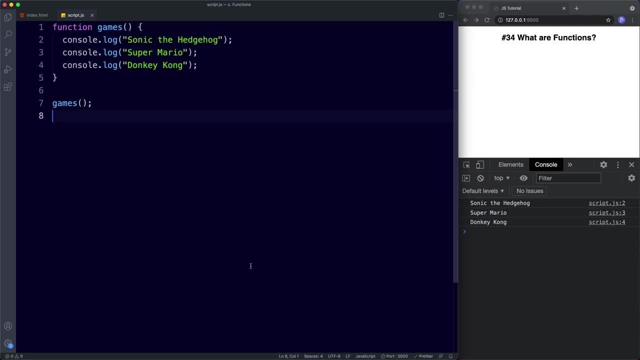 a piece of code, we don't need to keep rewriting it over and over again. We can simply invoke the relevant function and that code will run Now. another note about invocation is how functions can be invoked. Here we've simply invoked our function manually, but the real beauty of functions is that they can be called dynamically. 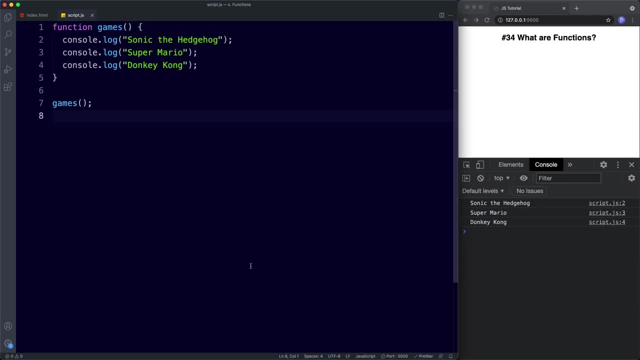 In other words, we can call functions based upon the user's button clicks or when the page loads, when a user hovers over an element, and much more. These are known as events, and we'll be looking at events in detail a bit later on. So, as mentioned, then, when it comes, to invocation, it's important to note that we're going to be looking at events in detail a bit later on. So, as mentioned then, when it comes to invocation, it's important to not be looking at events in detail a bit later on. So, as mentioned then, when it comes to, 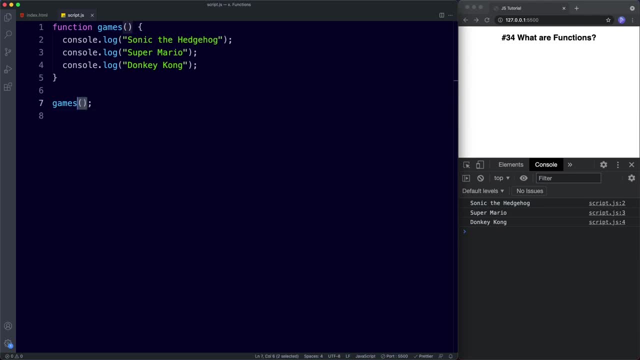 invocation. it's important to not be looking at events in detail a bit later on, So that we need the parentheses to invoke the function. As we saw, calling just a function name on its own simply refers to the function as a whole and does not run the function. So let 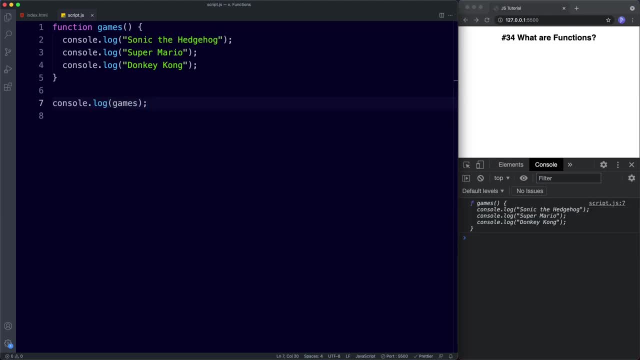 me show you that by console logging games like this In the console we see a reference to that function. F is the function. We have the name of our function, the parentheses and our code block. Let's talk a little bit more about what we can actually include inside of our function. 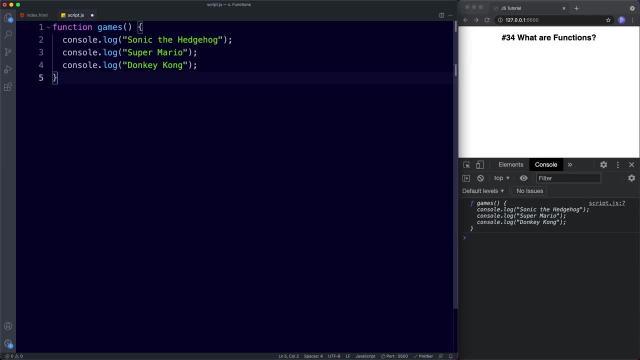 Remember, a function is simply a block of code that we can call or run. So anything we can write outside of a function, we can write inside of a function. so we can also create variables inside functions. so let's just go ahead and do that. so let's get rid of all this and instead we're going. 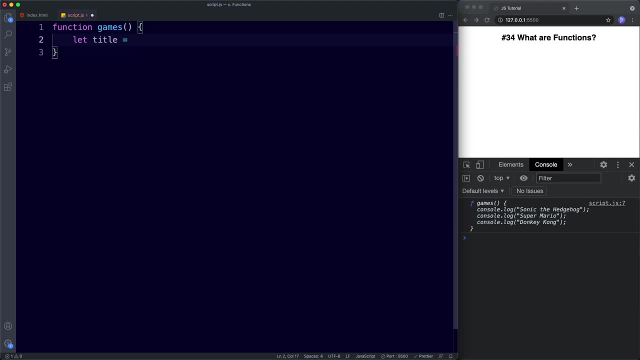 to say, let title be assigned the value of, and this time let's just go for zelda. and now we can consolelog our title variable and if we call our function again we can see we get zelda in the console. so this variable here is known as a local variable. in other words it's local to this. 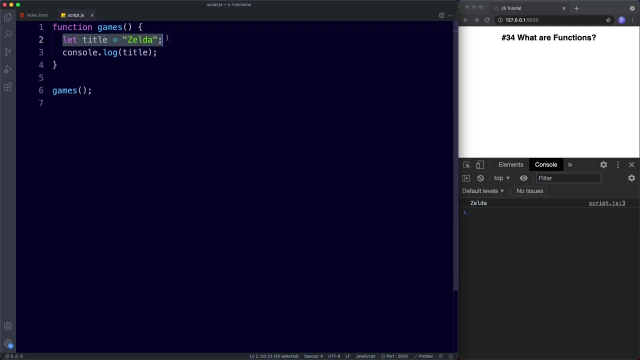 particular function. local variables are only visible inside the functions that they've been created in. so, for example, if we tried to consolelog title outside of this function, so we're trying to use this variable now outside of this function block. let's save. the console gives us an error. 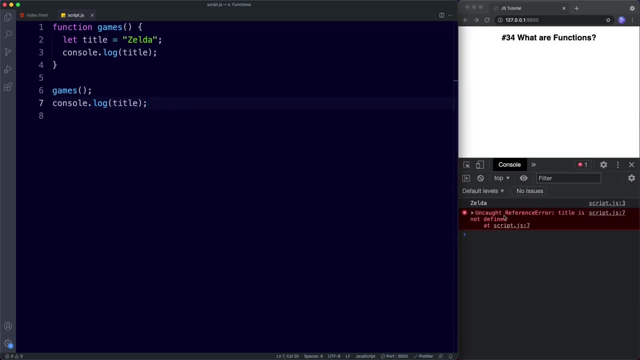 it says: unquote: reference error: title is not defined and once again that's because any reference error is not defined. so if we try to consolelog title outside of this function, variables that are declared inside of a function block are restricted to being usable only inside of that function block. we can't use them outside of the function block. so once again, this is known. 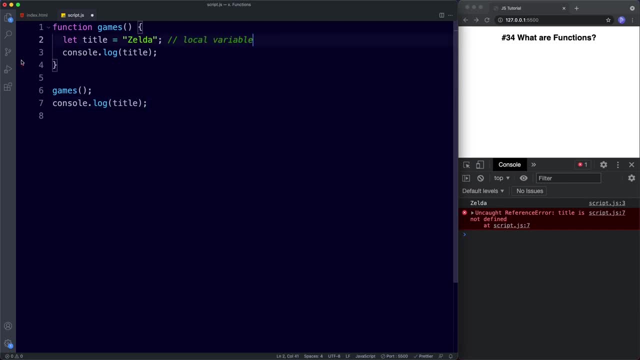 as a local variable. now, any variable declared outside of a function block, or any other block for that matter, is known as a global variable. so let's just put this above the function call. doesn't really matter where we put it. let's just say: let greeting be assigned the value of 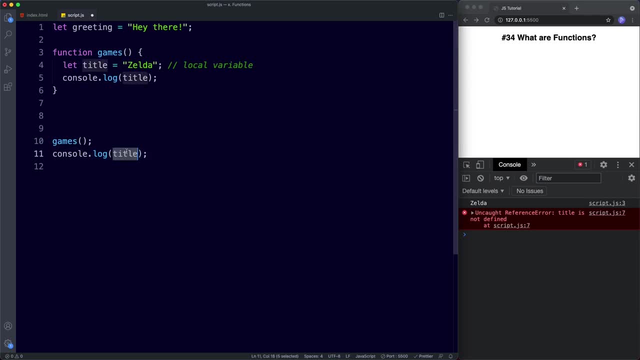 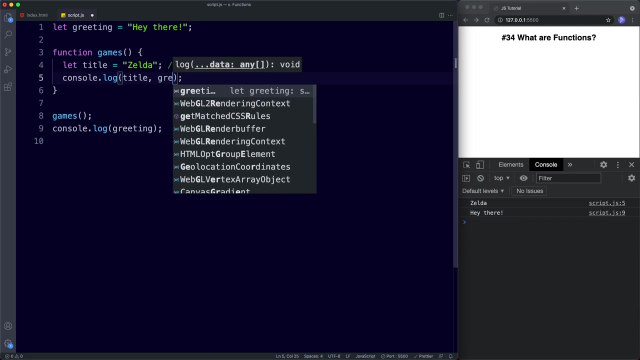 hey there and then down here that's consolelog greeting. let's save and we get hey there in the console so we can use this variable because it's a global variable and so since it's global, it's accessible globally or everywhere. so we can even include that variable inside of our function. save this and we get zelda. 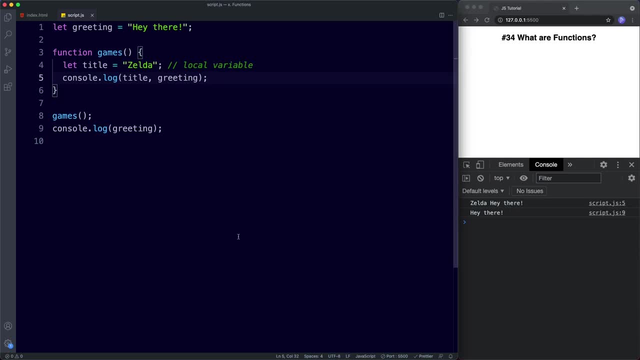 and hey, there now all this. so local variables and global variables. let's just put quick note in here: global variable- this is all to do with something called scope. we'll look at the specifics of scope in a few lessons time. we'll dedicate a whole lesson to 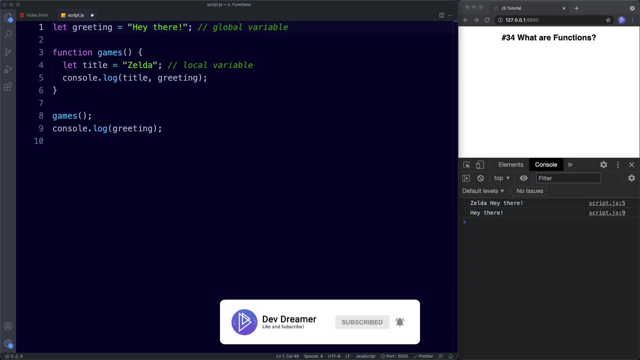 it because it is very important, but for now, i just wanted to introduce you to it so you understand how variables work when it comes to functions. now, functions can also be anonymous, that is, without a name. so up here, let's just get rid of this for now, and i'm going to say: let button be assigned. 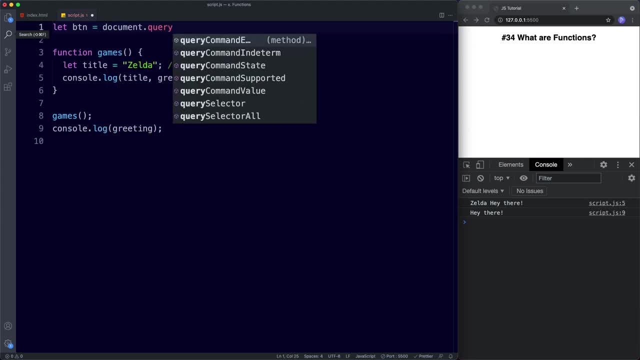 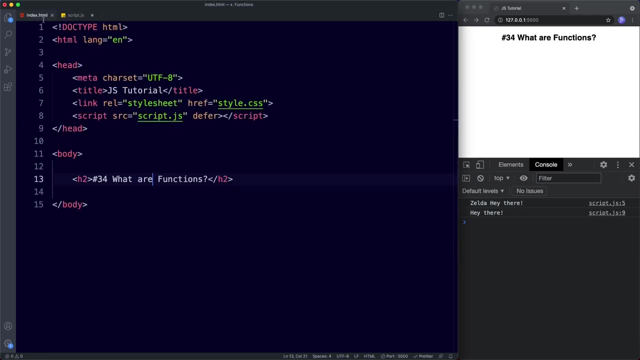 the value of document dot query selector, and what we're doing here is we're working with something called the document object model, or dom for short. we'll be learning all about the dom in future lessons, but for now what we're doing here is we're trying to select something from our document. so if we go to our indexhtml file you'll see we don't. 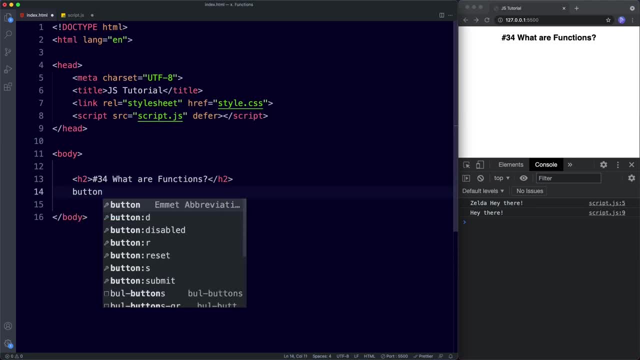 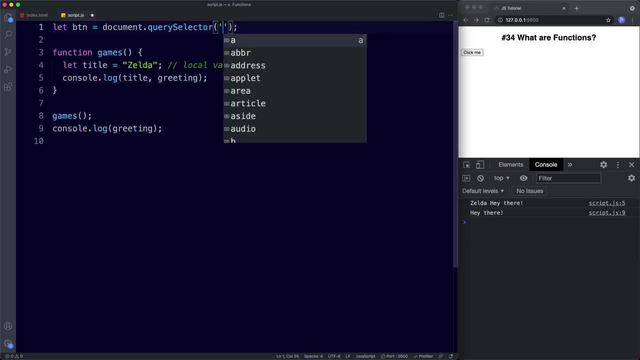 have anything here apart from the title. so down here i'm just going to say button with an id of button and we'll just say: click me. okay. so we've got a button and now in here in single plots we can reference that, just like we'd reference this in css. so i'm going to say hashtag button. okay now. 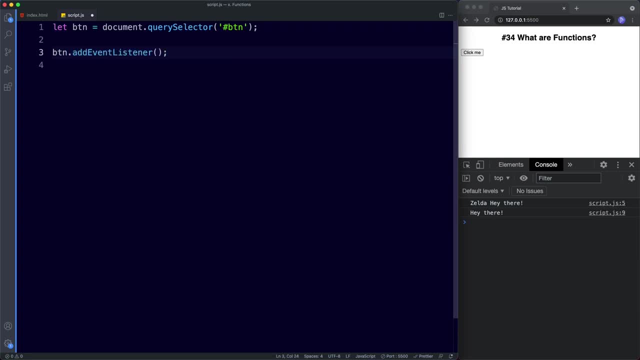 what we're going to do is we can say button dot, add event listener. so we mentioned events very briefly earlier on. these are things such as click, hover over, etc. etc. what we're doing here is we're saying: take this button- which is a reference to our button right here- and add the event listen to. 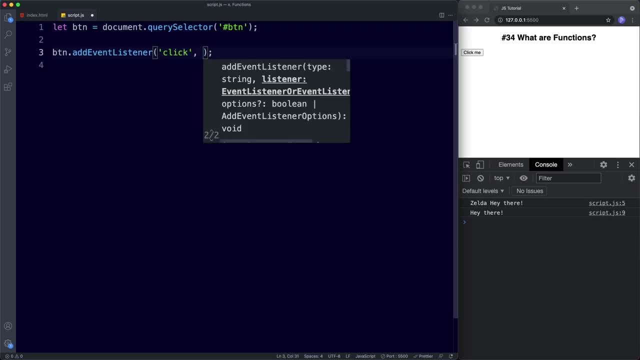 it of a click, so we say comma. and here now we actually have our function. so i'm going to say function as mentioned. we don't need a name, we don't need any parameters. we'll look at what that is a bit later on. we've got our curly braces inside here. 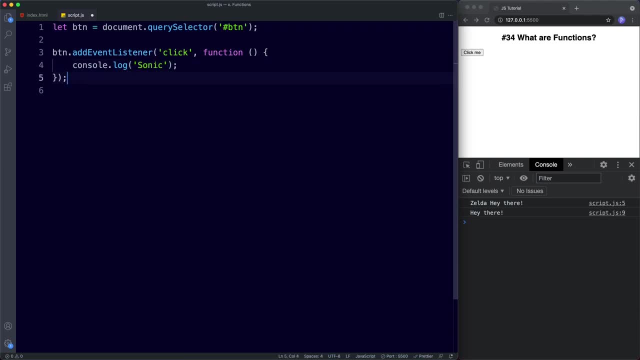 so log sonic. so what we have here, then, is we have an example of a function. okay, this, right here, there is right there, it's exactly the same as the other function we looked at, except it doesn't have a name. you'll see why in just a second. so what we've done here, then, is we've created a button. 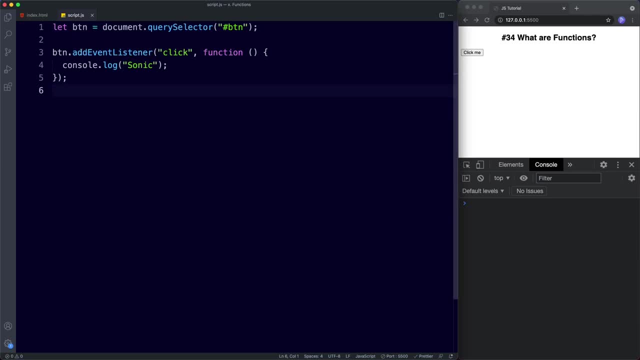 we've created a reference to that button, stored it in the variable btn or button, for short. we've then added an event listener to this button of a click. so when we click this, we're going to do something, and that something is this function here, this anonymous function. we call it an anonymous. 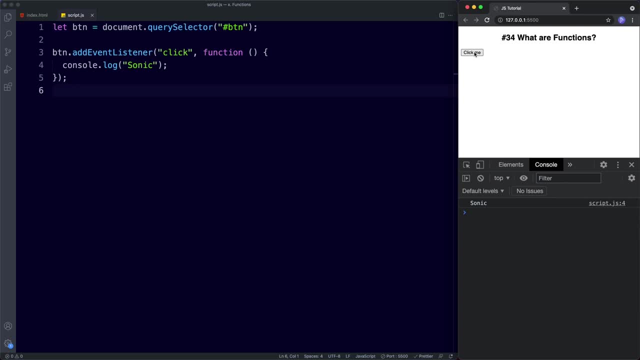 function because it doesn't have a name. so if we click this, we get sonic in the console. if you keep clicking it, we'll get multiple sonic calls in the console. so the point of showing you this- i know it's stuff that we haven't actually looked at in detail right now- we will later on- but the point of showing you this is that we can. 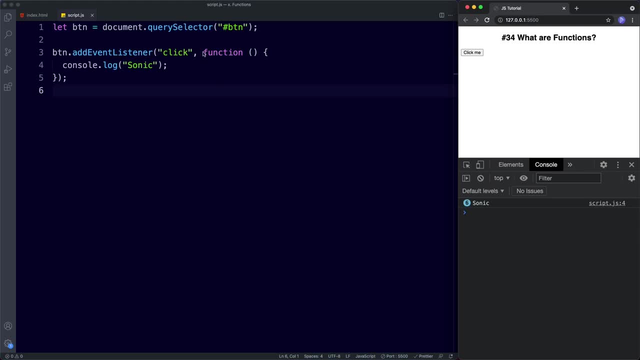 have functions that don't have a name. the only way for this type of function to be invoked is by an event handler. however, there is a way that we can create an anonymous function and still have a way of referring to it in our code, and that's by using a function expression. we'll look at function. 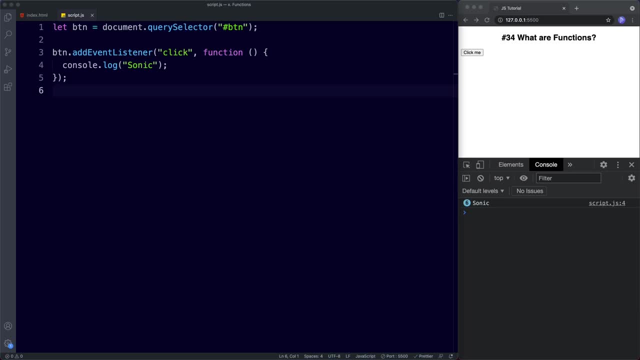 in the next lesson. so, guys, that's all about an introduction to functions and how to write functions by using function declarations. as mentioned, the next few lessons will be all about understanding functions, as they really are a major part to mastering and understanding javascript. for now, let's go ahead and summarize this lesson and let's just put our original. 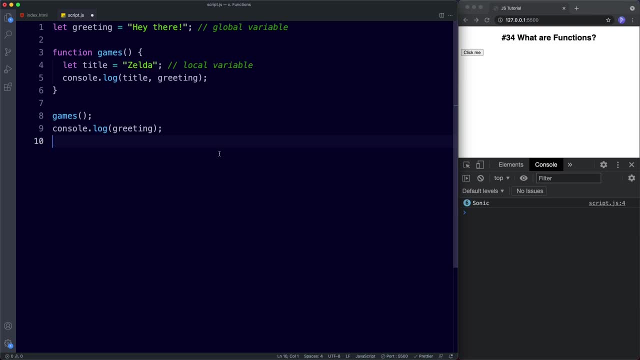 function that we had on the screen. so functions are blocks of code that we can call or invoke whenever we want. we saw that there were four main ways to create a function: function declarations- and we've covered declarations in this lesson. we'll look at expressions in the next one: arrow functions. 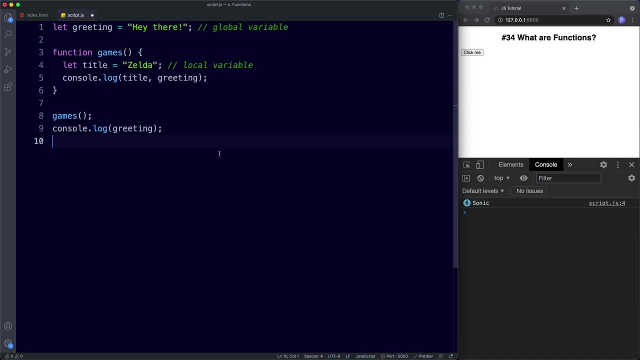 constructor functions and generator functions. to create a function declaration, we simply use the word function, followed by a name, parentheses and then finally curly braces, and it's inside these curly braces that our code to be run is placed and finally functions on their own, do nothing. they need to be invoked or called in order for the code inside the function block to actually run. the 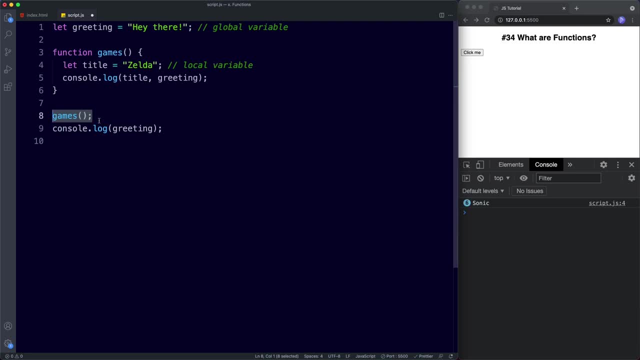 functions is by using the function name followed by parentheses. okay, so let's take a look at your tasks for this lesson. for task number one, i want you to create a function using a function declaration called my name and then invoke the function to log your name to the console. 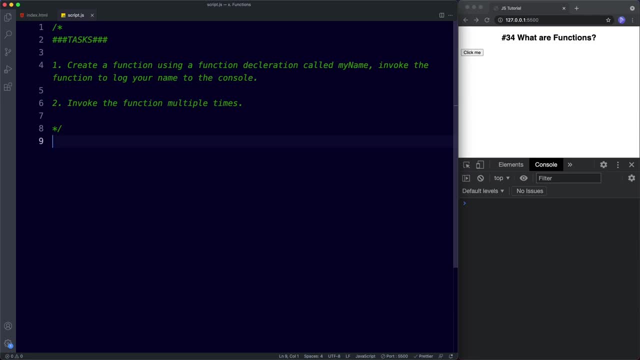 and then for task two, i want you to invoke the function multiple times. so it should be nice and straightforward. go ahead and pause the video, try this out, and when we come back we'll take a look at the answers. okay, so how'd you get on then? let's see. 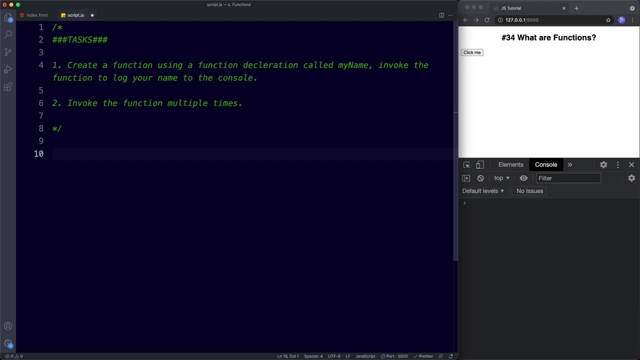 so for task number one, we need to create a function using a function declaration. so we use the keyword function and this function should be called my name. so we say function space, my name. then we need a parentheses, very important. we need a parentheses after the name space curly braces. so 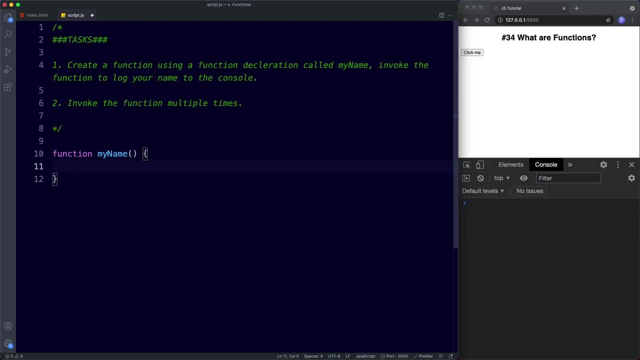 this is our basic shell for our function. inside this we need to consolelog our name. so i'm going to say consolelog and then my name, and then for task one we need to invoke this function. remember, our function is by using the function name, so we're going to say my name and then, very importantly, 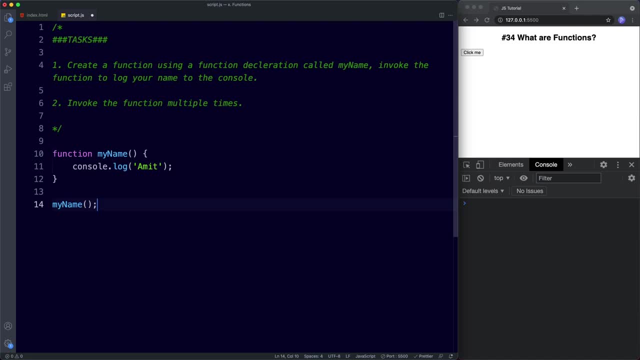 include the parentheses at the end. so let's go ahead and save, and, sure enough, we get amit printed to the console. okay, so that should be nice and straightforward. and then, for task number two, we need to invoke the function multiple times. so again, nice and easy. all we need to do is call.